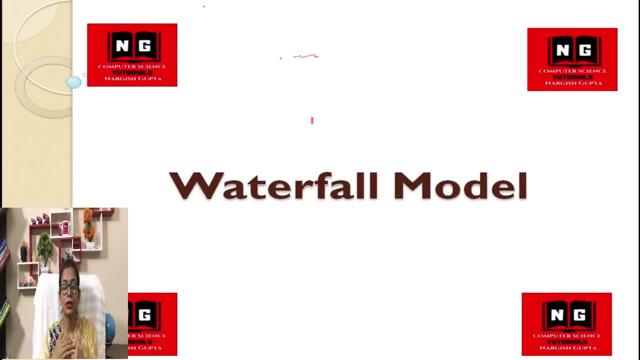 which is flowing from top to bottom, So there are no chances that the water flowing from top to bottom, So there are no chances that the water flowing from top to bottom, So there are no chances that the water flowing from top to bottom can be back. So there is also same with this model. 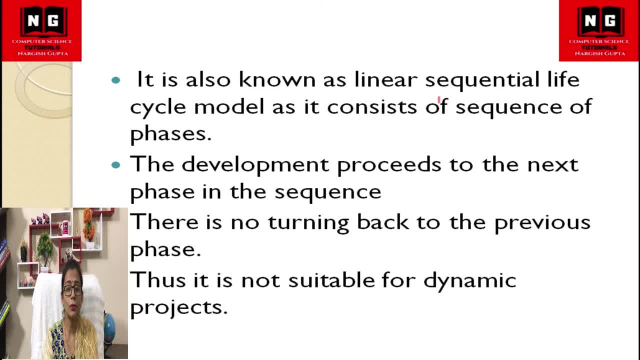 We also call a waterfall model as linear sequential model. We also call a waterfall model as linear sequential model. Why are we calling it as linear sequential model? because it consists of software development life cycle phases: step, step, follow karenge, aur ek sequence mein, follow karenge. there will be no turning back. 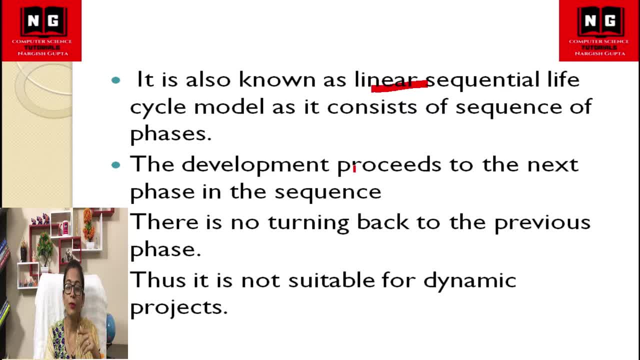 jaise ki. second point: bolta hai, kya bol raha hai? maara ki the development proceeds to the next phase in the sequence, same sequence mein. hum follow karte jayenge har ek phase ko. there is no turning back to the previous phase. there is no turning back. this is the. 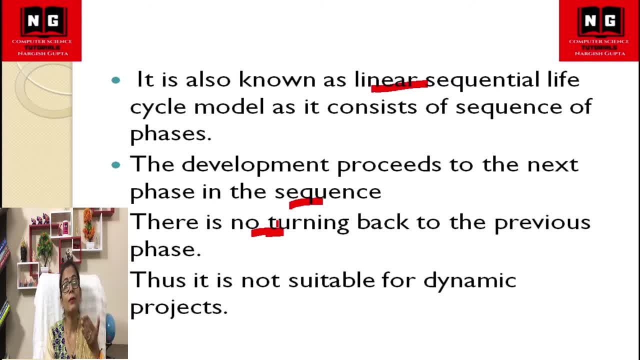 main point for waterfall, that is ki, agar humne ek phase ko complete kar liya hai, there is no turning back to that particular phase. means, agar suppose humne requirements ko apni gather kar liya hai and srs humne prepare kar liya, aur uske baad hum design phase pe. 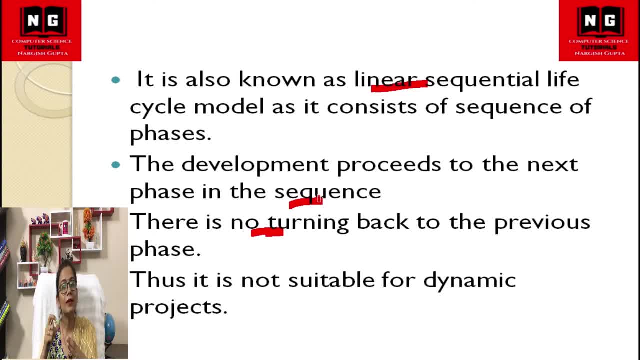 move kar gaye, aur design phase pe aane ke baad humne lagta hai, ki nahi yahaan pe requirement mein kuch disturbance hai. to hum wapis requirement phase pe nahi ja sakte. ye ek is waterfall karte hai. 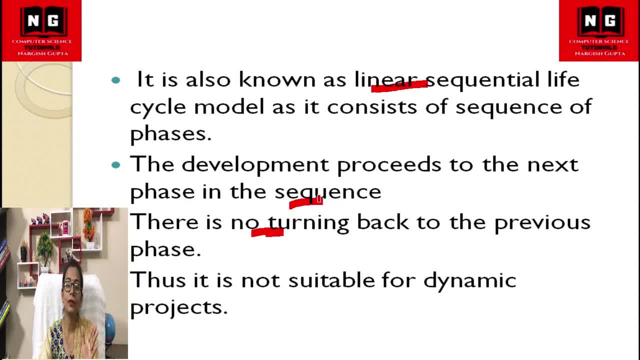 waterfall model ka sabse bada point hai ki there is no turning back to the previous phase now. the last point is thus: it is not suitable for dynamic projects. so dynamic project ka matlab kya ho gaya jahaan pe cheeze continuously, aur we can say somehow: kahina, kahin, kuch, kuch. 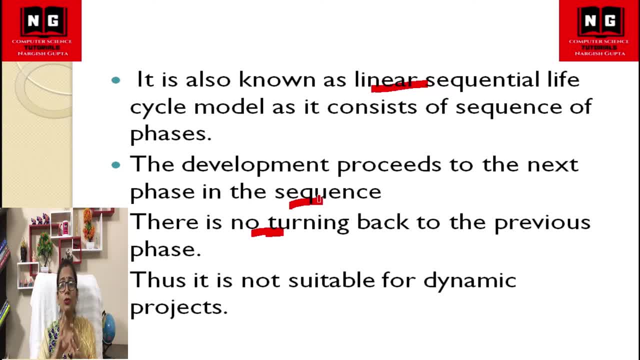 cheeze change hoti rehti hai, toh vo hota hai. dynamic projects, toh jo ek stable project ho, jiski requirements hume achche se pata ho, sab kuch fixed ho. usi mein hi water fall model use kar sakte hai. 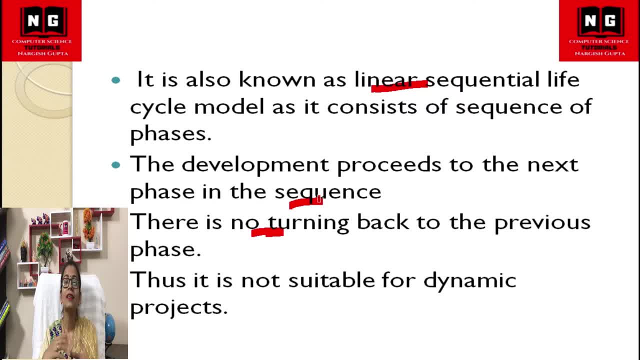 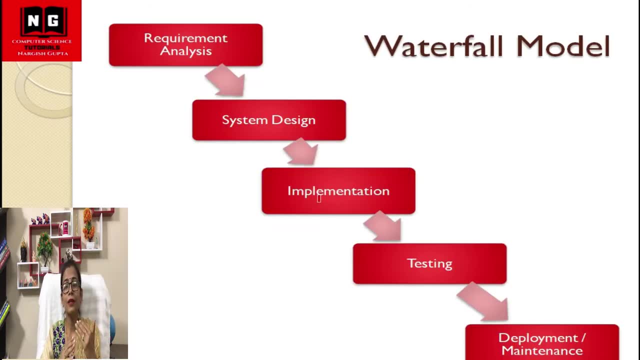 waterfall model ko hum classic model hay. kyun ki yeh sabse inial model hai. yaha basic model hai amare software derivelement life cycle ka. ab hum iske diagram pe ayajte hai digital main khya batara hai yeh amare phases batara. 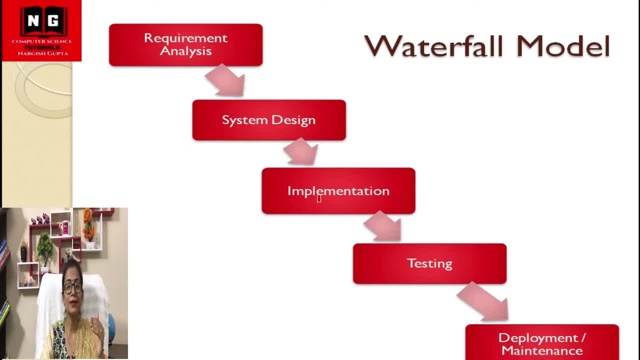 hai waterfall model ke toh. so we can see that is the anytime: phthis, wetar, f, CSS requirement analysis, system design, implementation, testing, deployment and mentaffe. So we can see what are the phases: Hattish requirement analysis, system design, implementation, testing, deployment and maintenance. So now we will discuss our once cái. what are Currently say out of it in our defens, where what start at RC overlap a camera prong one twenty to come and they will not encounter much image painting and kaliyen, all the stages like of Hai Freropy by phul. 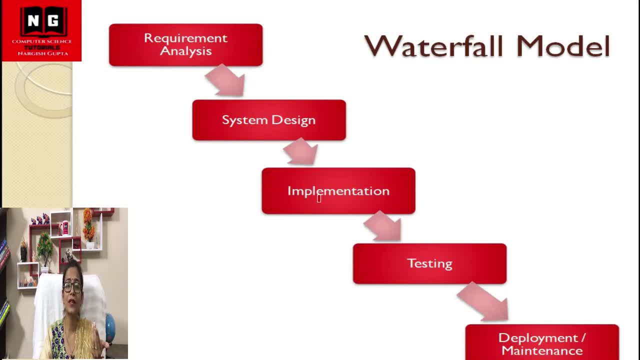 So our first basic model is our basic model. we are takes here process, they the background model. so we have defined the design is: Do you have a lot of this component maintenance. When we studied software development life cycle we studied the same phases but before requirement analysis we had kept planning. So in planning we had 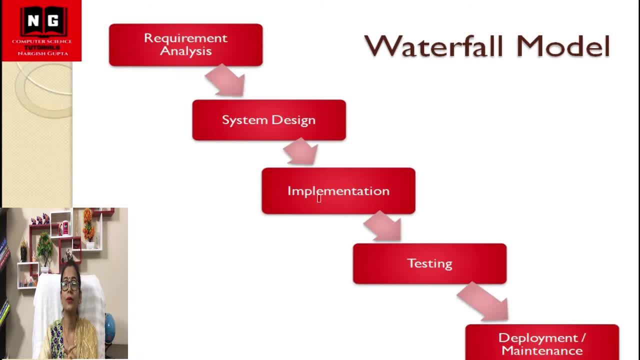 discussed at that time that what we are basically doing in planning we were deciding how to allocate resources and how to plan all the things. do we have to move forward with that project or not? that means we are checking the feasibility of the project. So that thing happens in our planning. 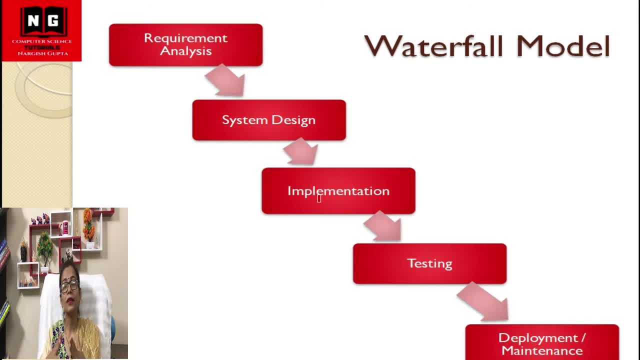 After checking that feasibility we decide which model we will take with the project. So the planning phase is already covered in which we decide which model we will take. so suppose we have decided that we will take the waterfall model for our particular project. 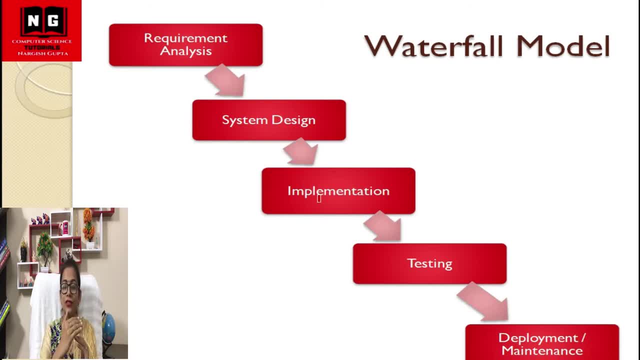 So when you come to the waterfall model, then our planning phase is skipped. So we start here The requirement analysis phase. so what we will do here in the requirement analysis phase is that whatever project for which we have decided that okay, we will going to work on this particular project. 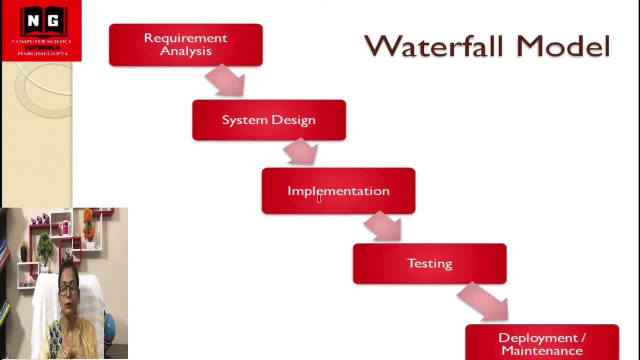 then we will start gathering the requirements for that. there are different, different processes of requirement gathering and of analyzing the requirement By including those processes and gathering the requirement that, Okay, this particular button will be here, that so many number of pages are going to be done. 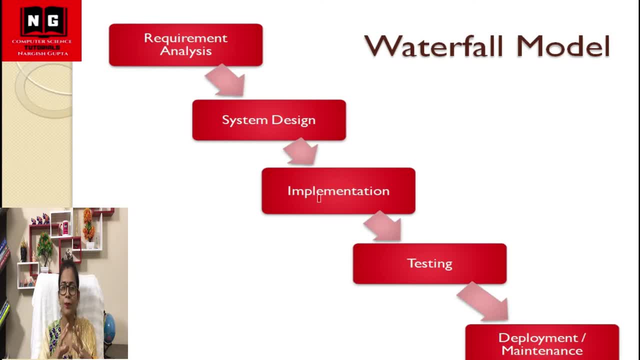 so many clicks are going to happen. we have decided all these things. after analyzing the requirement, we will come to the next phase, that is, system design. we have come to the system design phase and when we had studied SDLC, we had seen that when we do requirement analysis, 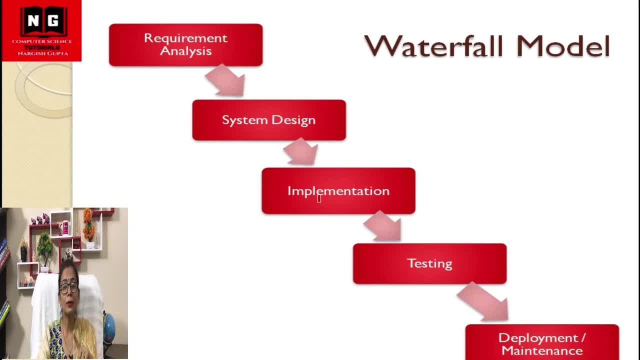 we get a document after preparing. what we used to say is SRS. so from here, what document we used to get SRS, we got SRS. so now here in waterfall module, the biggest thing is if we made SRS here, then it will be fixed. now we can't change it. 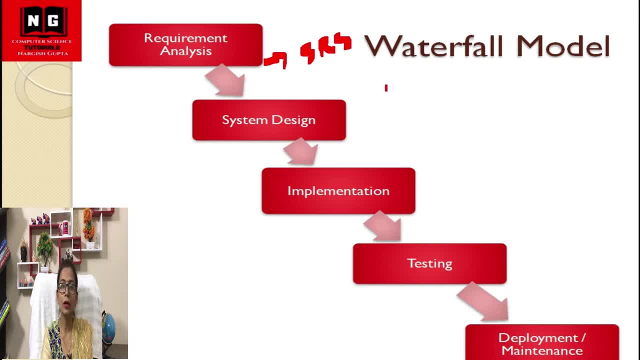 now we have to move forward in the flow because this is the process of waterfall module in which we can't do turning back in our phase. so our SRS is prepared. after SRS we will come to system design phase on system design phase. according to that SRS, 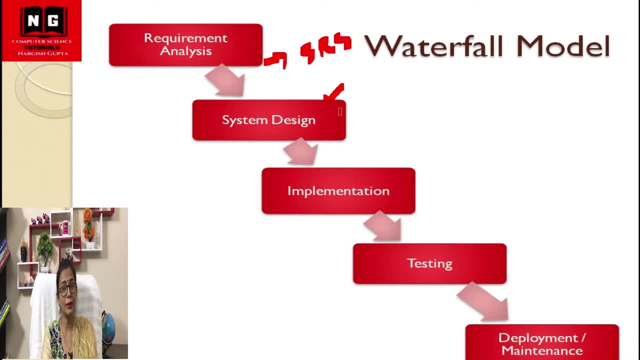 we develop our design means we make a blueprint for our projects, means the particular software we are going to make. we make a software blueprint and prepare a document. what comes here, design document comes here. design document is also fixed here. after fixing, next we go to implementation phase. 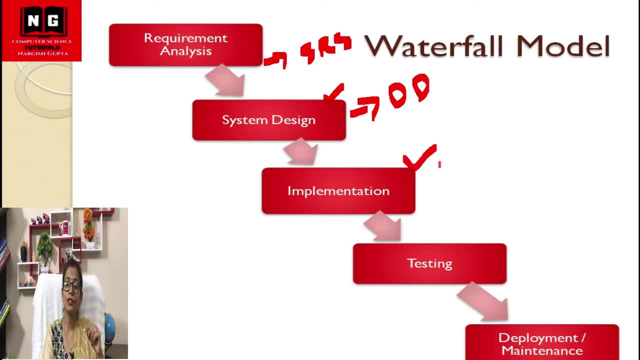 when you come to implementation phase. so in implementation phase we will implement using both the documents that we have made. we are doing implementation but even after coming here, if we feel that there is any issue or any risk, then we cannot go back the same- both the documents. 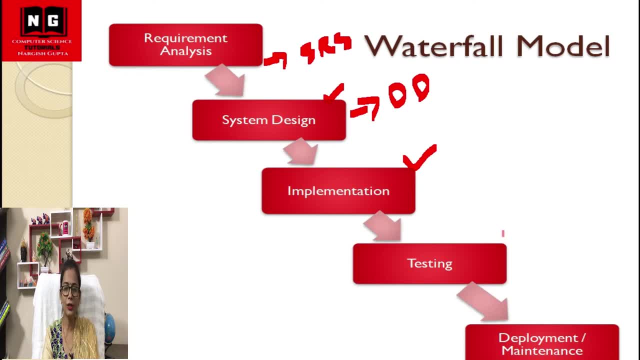 whether there are errors or risk. then also we have to move forward. after coding implementation we will do testing. in testing we get flaws. we have to complete that particular project with those bugs. only after testing we deploy. this is our whole process of waterfall model. this is the process. 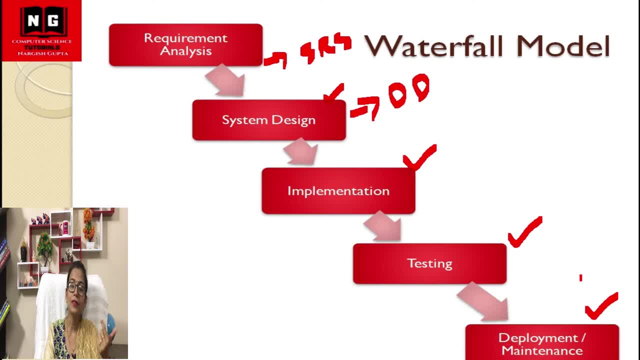 and the biggest issue, which I am saying again and again, that we cannot go from any particular phase to another. so this is our flaw of waterfall model. that is why it is said that we use waterfall model there which are small projects, or in such projects whose requirements are fixed. 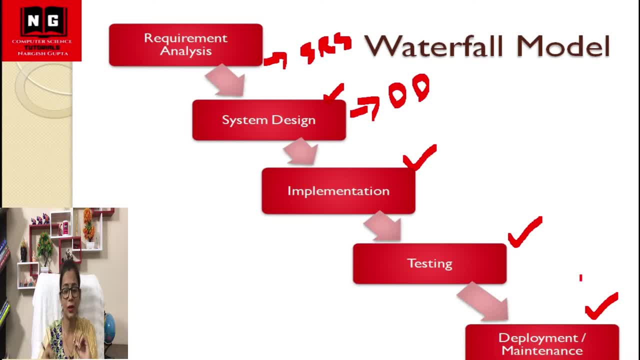 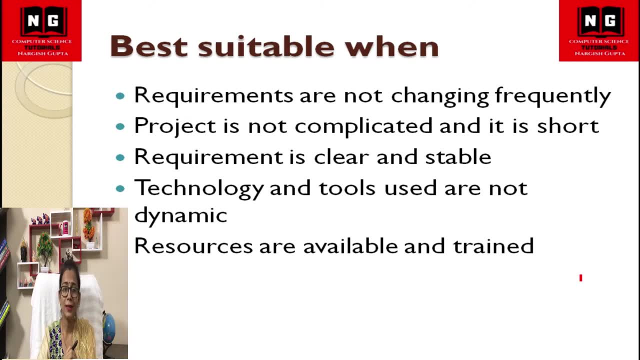 means there is no chance from anywhere that we change it. so let's see it is best suitable when. so the waterfall model for what type of projects or for what time will be best suitable? we are discussing those points here. so, first of all, our requirements are changing frequently. 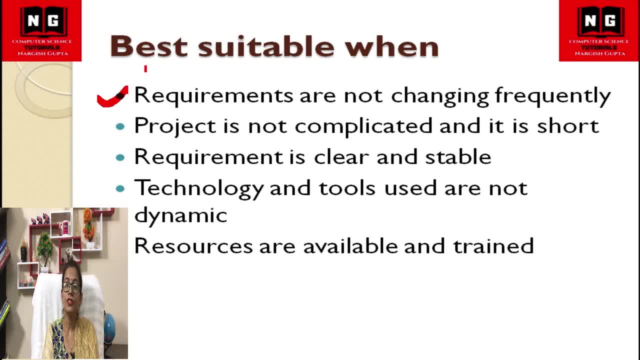 not changing frequently means stable means for the project, whose requirements are stable. for those projects, waterfall model is best. now coming to the second point, that is, project is not complicated and it is short means it is simple and small. project that's it. requirements are same point. requirement is clear. 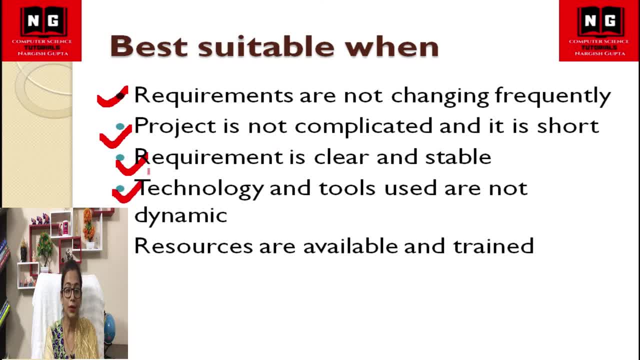 and stable and tools are not dynamic means the technology which we are using should be fixed. it is not like that, that now we are working in particular technology and after taking it half way we feel, no, not this, we should move on some other technology. so, basically, if we are using 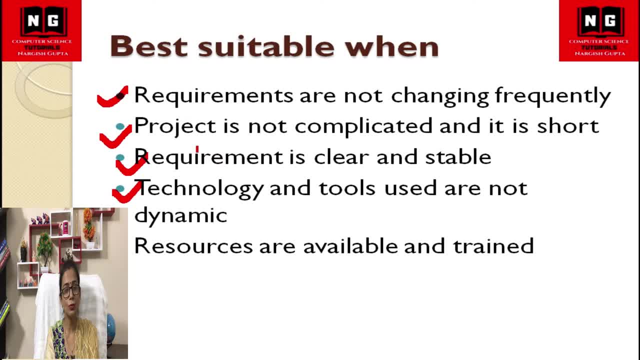 waterfall model in any project, it means that all the things of that model are already fixed, be it resources or our technology or requirements. everything should be fixed. there should be nothing which is dynamic in this project. now the last point, which is: resources are available, and trained means. 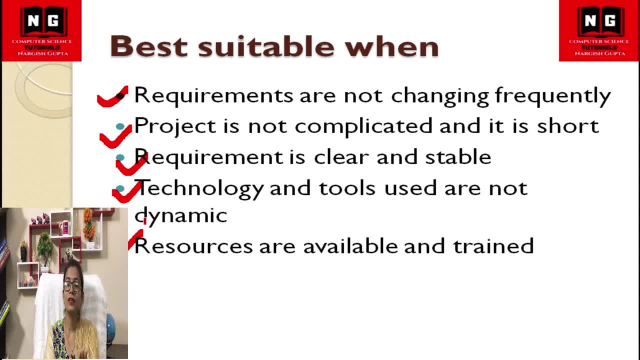 we don't have to worry about resources. all these things should be fixed in that type of project. we can use waterfall model. so when there is a model, there will be advantages and disadvantages of any model. so let's come to the advantages of waterfall model in the advantage of waterfall model. 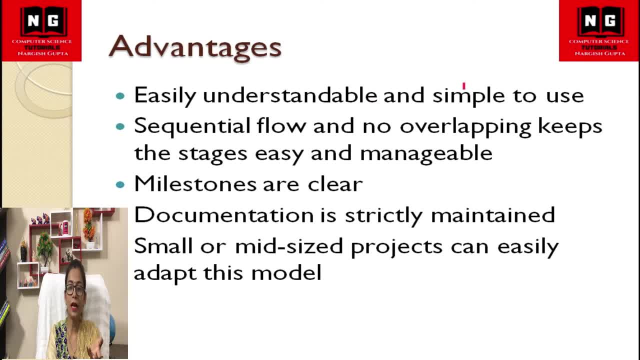 first point is easily understandable and simple to use. that is like: okay, sequential flow and no overlapping keeps the stages easy and manageable if we discuss this point. so what he is trying to say, the advantage of this, is that we are doing a sequential flow. sequential flow means waterfall. 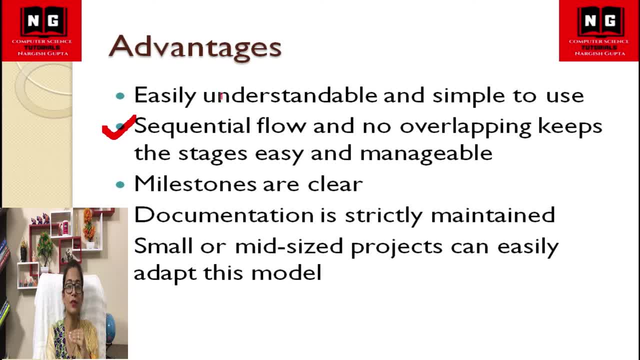 we are following step by step and in a sequence. we are following all the phases and there is no overlapping means there is no option to go from one phase to another. so what is happening is we have managed every stage very well. the output of every stage will be fixed. 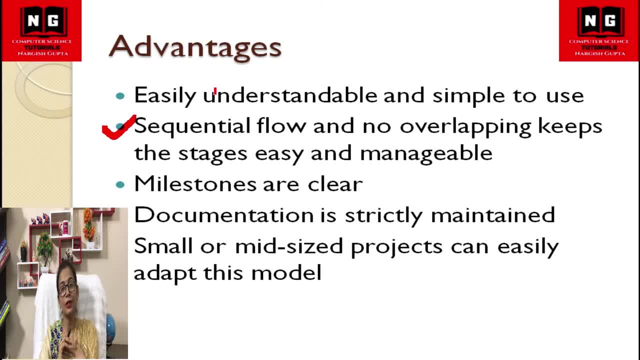 and our proper documentation will be maintained very well. why? because we are not like going to the next phase and then coming back and then doing some changes. so because of this there are chances of ambiguity. but there will be no such chances because if the document is made, 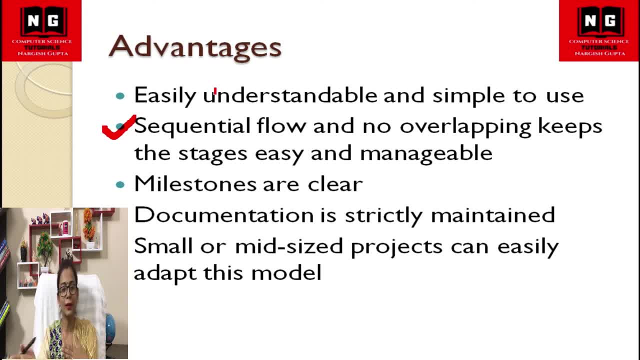 then it is made. if we get out of any stage, if we get out of a particular phase, then it is out now. milestones are clear means we know that we will get this thing from this phase. so milestone is clear. that is why we are getting maintained, because we are not going back and forth. 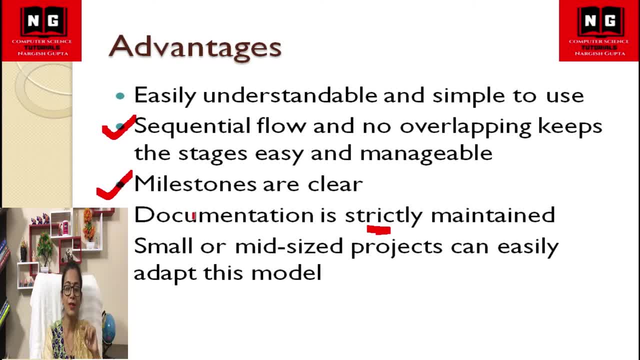 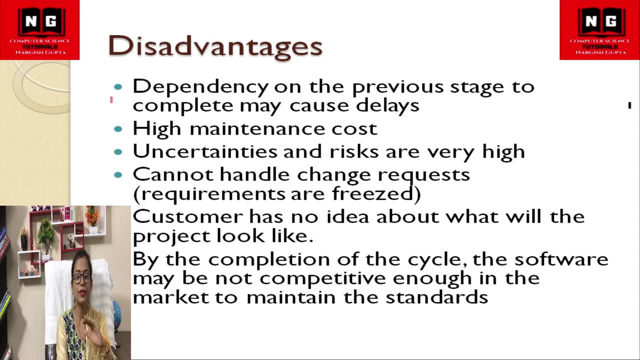 now. it is good for small, mid size project and can easily adapt this model. so these small and mid size projects, they can use this model very well. now come to the disadvantages. we have seen the advantages, now let's come to disadvantages. the first point is dependency on the previous stage. 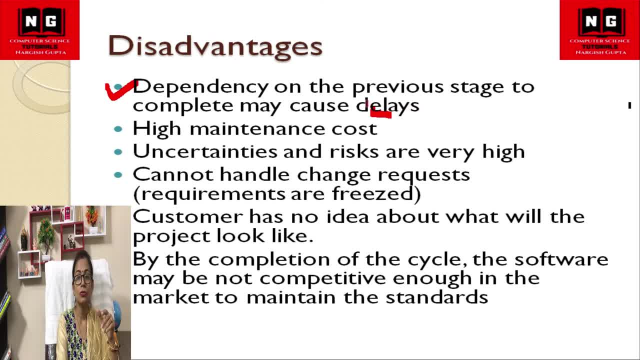 to complete may cause delays. so in our waterfall model, our dependency is on a particular stage. why? because until we complete our first phase, we can't go to the second phase, so this can cause a delay cause. if we want to understand it as an example that we are making a project, 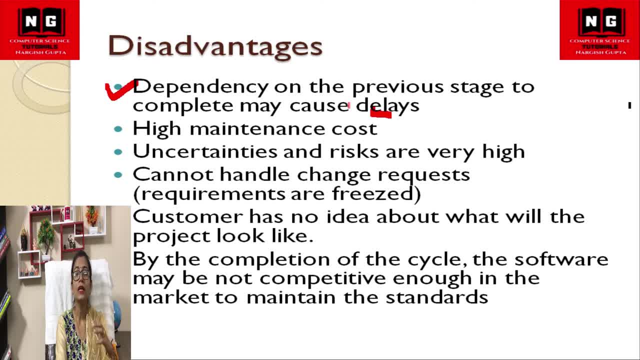 requirements analysis is done, system designing is done, come to implementation and suddenly, for some particular reason, we are taking time in implementation more than expected time. so due to that, our project will get delayed. why? because in implementation we took more time. after testing and testing, our deployment will be delayed. 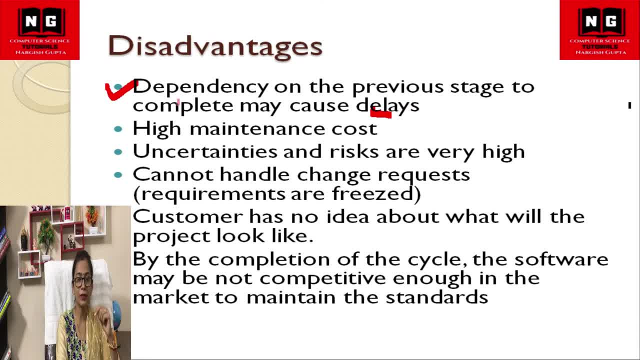 so this is a big issue that, due to previous stages, it can be delayed. next is high maintenance cost. why high maintenance cost? because whatever project we have made in between any risk or any issues, to debug them, to fix them again, we have to do renovation in the whole project. 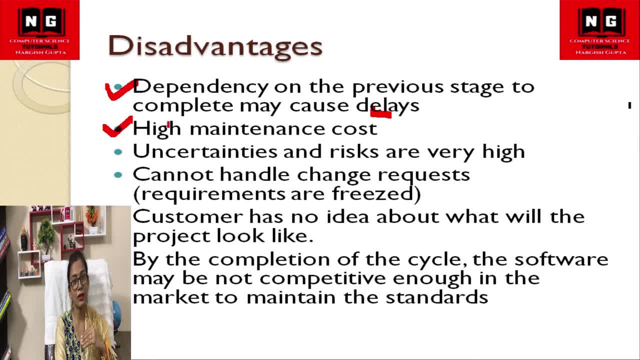 or we have to bring changes. for that we have to start phases again, so thus it will going to cost high. there are uncertainties, risk are very high because we don't know we are making the project. everything is going fine, but sometimes there are chances that changes come in different market. 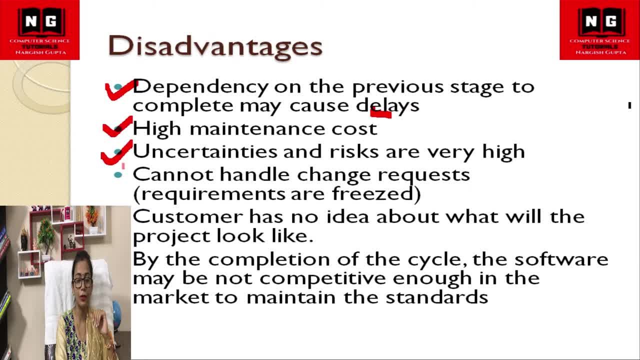 but it can deal on risk. our particular project cannot handle change request. now, whatever our customer was, he gave us the project. he gave us the project, thinking: ok, fine, according to his requirement, all the things will be done. but later, in the middle of the development of the project, 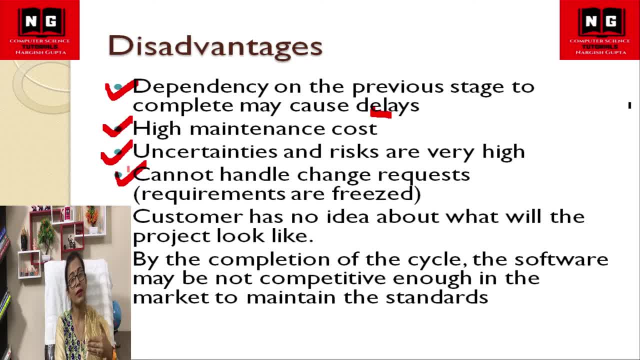 he feels that this was another requirement. so now we will not be able to handle any requirement. so this is a point that we can't handle. any change request then comes. one customer has no idea about what will be the project look like, because the project that we are making 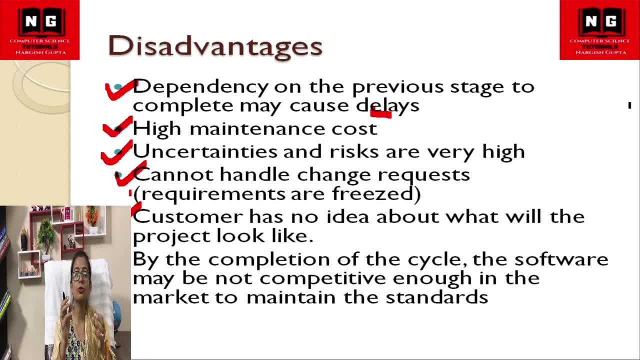 will come in front of the customer only when it will be complete. it is not like that we are making a particular part of the project, showing it to the customer according to his expectation or not. so this is a very weird picture for the customers that what to do. 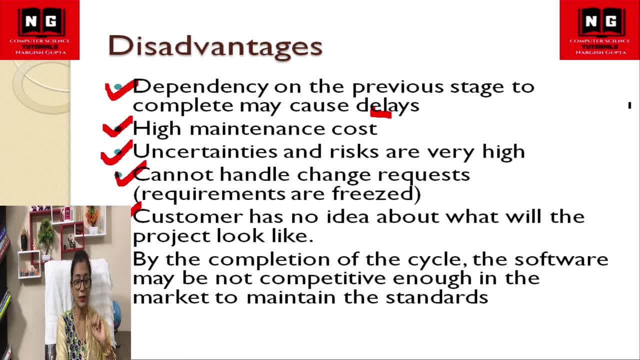 at the end. only we will know how the project will be made. now. the last point is by the completion of the cycle, the software may not be competitive enough in the market to maintain the standards. why? because we made our software and in that, the market requirements. there were some change requests. 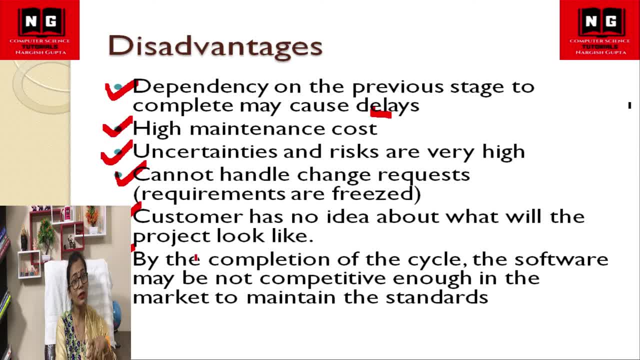 or there were some particular changes that needed to be done, but we could not do that. according to our old requirements we have developed our project. so thus that particular project that we have completed does not remain competitive because our change request does not exist in it. due to this, 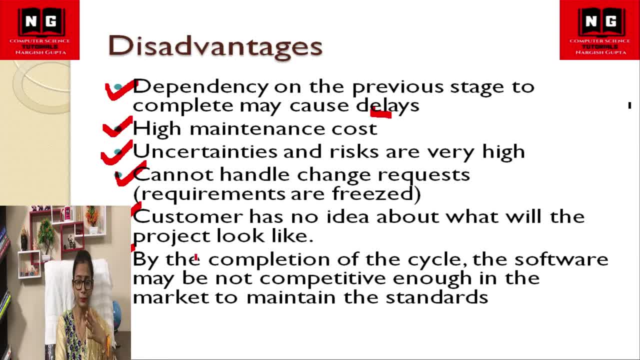 there are chances that it will not be competitive. so till now we have seen what is waterfall model, its diagram, the phases, in particular after that, its advantages and disadvantages, and where we can use waterfall model. so what we call waterfall model is a linear, sequential model and the main point is: 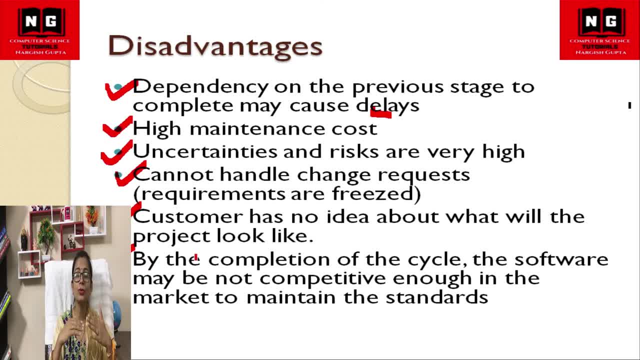 that we cannot switch from one phase to another means we cannot switch back. turning back because the flow of water is like this, so it is flowing here. there is no back option. so this was an issue due to which there were many problems, so to solve that, there is one modification. 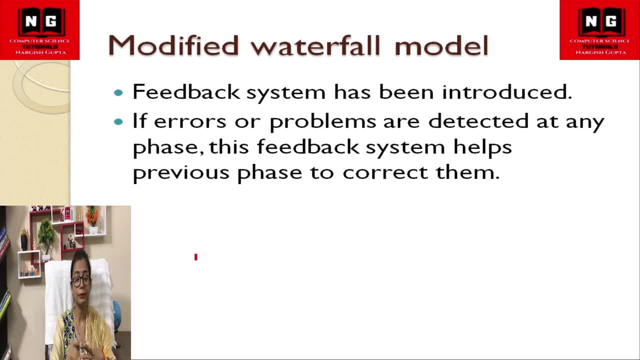 in waterfall model. now we will discuss that, what we call modified waterfall model. what we added in this? we used only one small thing: we introduced a feedback system. the feedback system that we introduced. what has happened is that our two consecutive phases- they can work according to feedback. 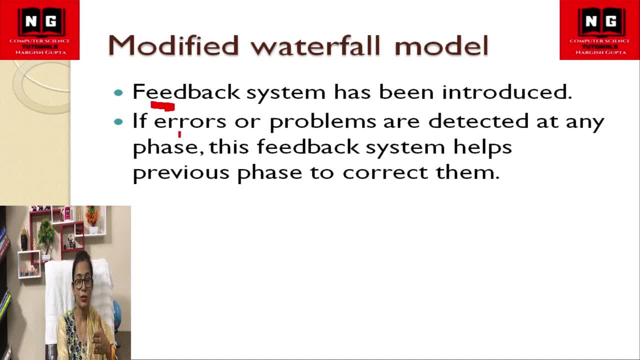 means suppose we reached testing phase and we got some bug. but our classic waterfall model- according to that we could not debug that bug- means we could not correct because we could not go back to implementation phase. that is why now this modified waterfall model has this feedback system. 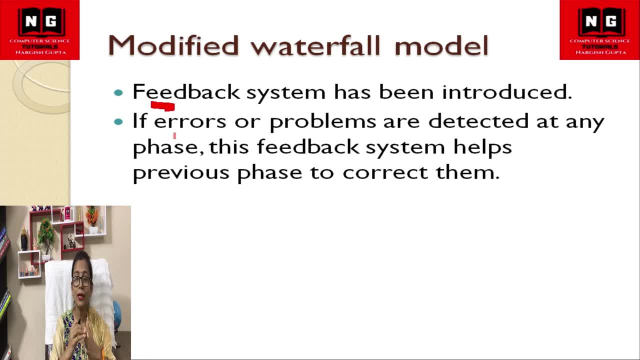 so when we went to testing phase, we got this feedback that there is one issue or two issues. so we can go back to implement phase and we can change. and the main point is, if errors or problems are detected at any phase, at any phase, feedback system helps. 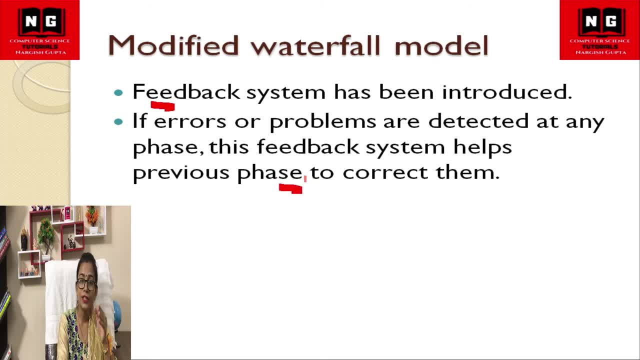 previous phase. to correct them means at any phase. if we get an error, we can go to previous phase and correct it. if we understand this with an example, what were our phases? requirement then: designing. after designing comes our implementation phase, implementation phase after testing, and after testing comes